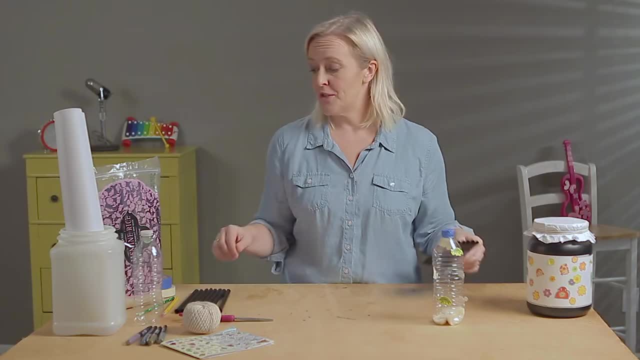 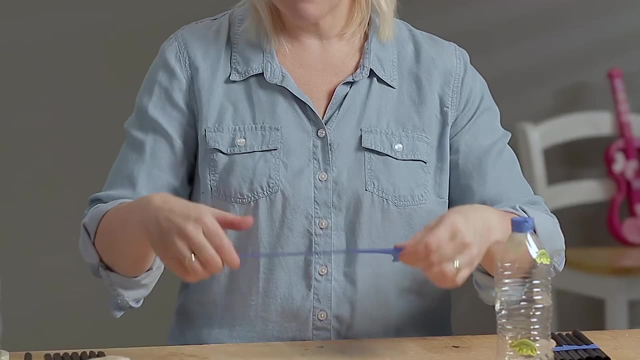 tape and some scissors. What you need to do for this is first get your piece of tape. I love using painter's tape because it is so easy for children. You can use masking tape whatever you have really, and I like to just fold the little ends under so it sticks. 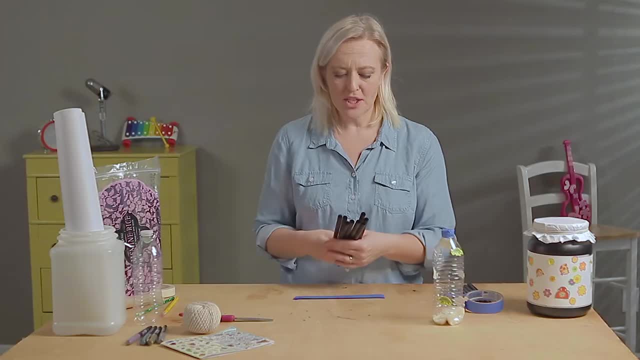 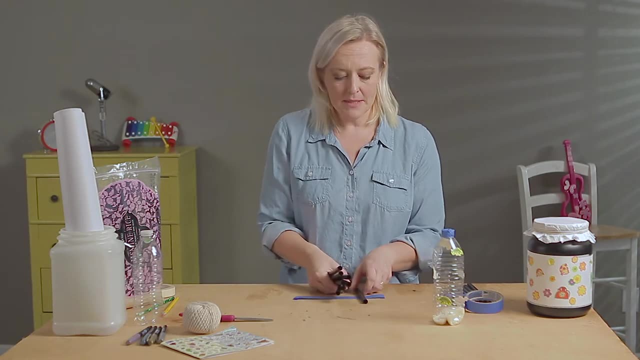 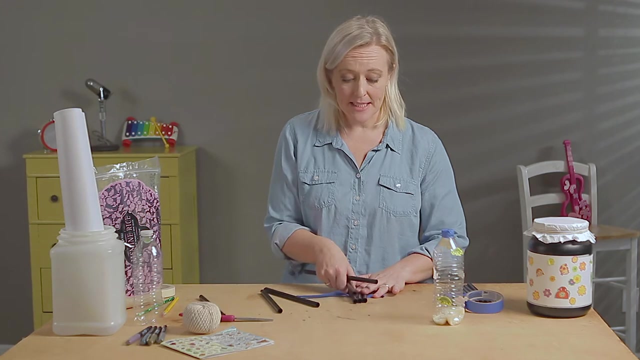 down. Now we're going to get straws. Now it's up to you. these are bubble tea straws, so they're nice and big, but you can just use normal straws and you want to lay them down across the tape and try to keep them, even at the top- Super easy. 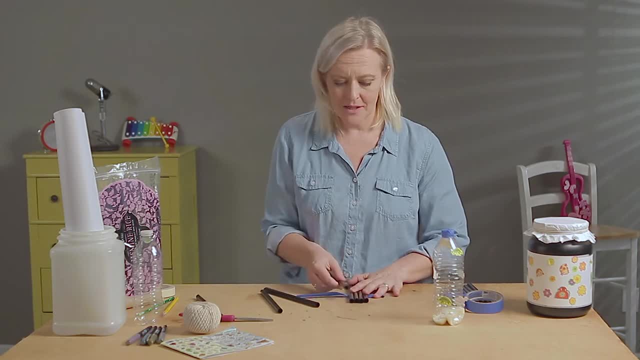 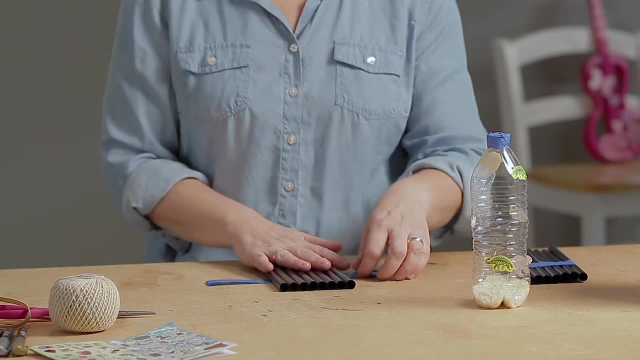 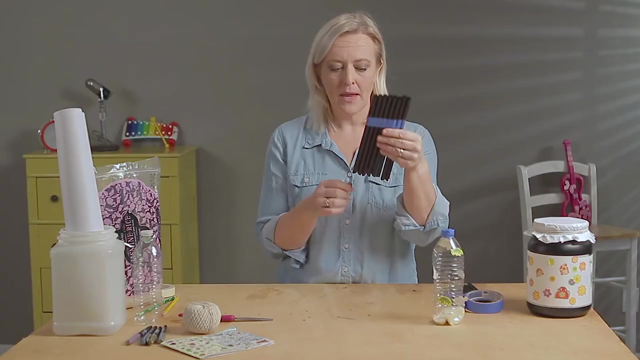 to do. your children can do it, even I can do it. So we're just going to stick it across the top of the tape and once you have that, it's a matter of picking up the ends of the tape and folding it back over. There we go Now, what we want to do. 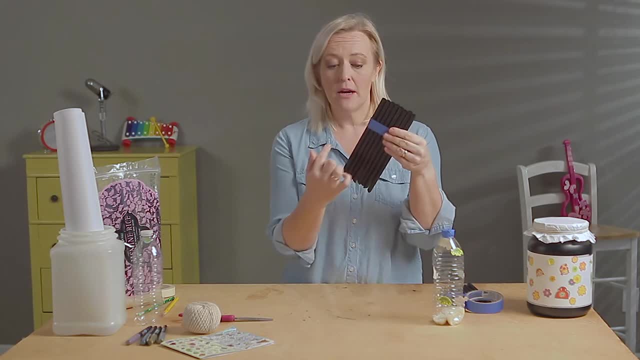 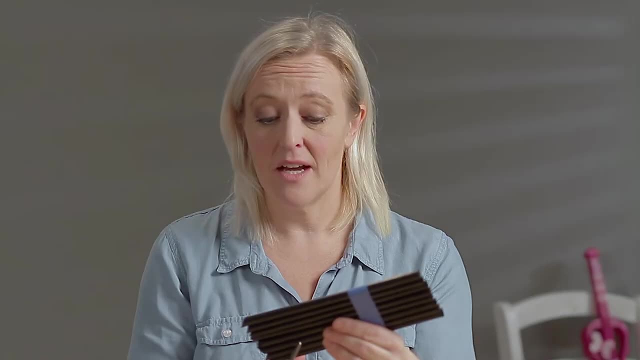 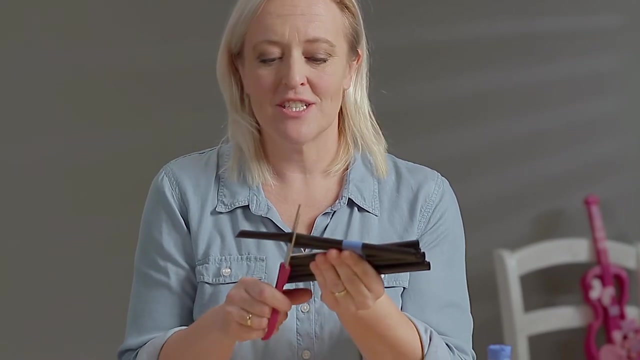 is make. cut the bottom and with a pan flute they are always staggered. Now you could try to cut each straw first and do them differently. no, no, no, this is the easiest. cut across the diagonal And your children can do this. straws go. 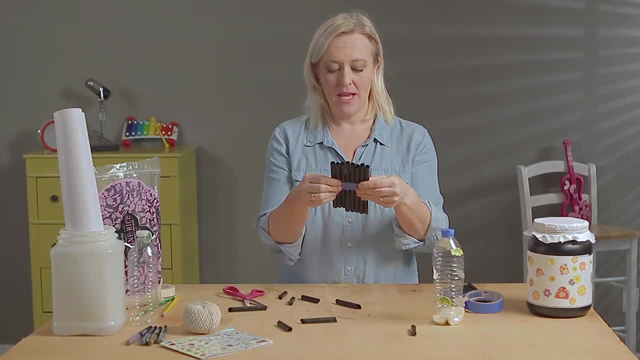 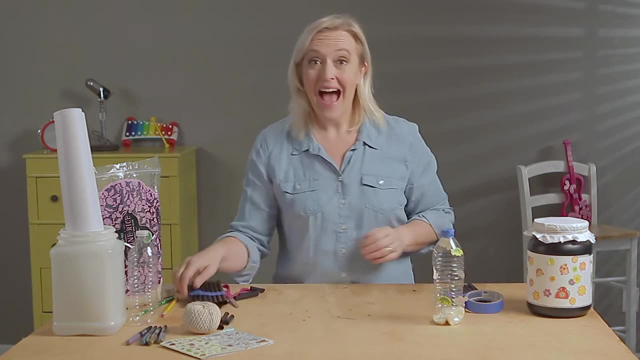 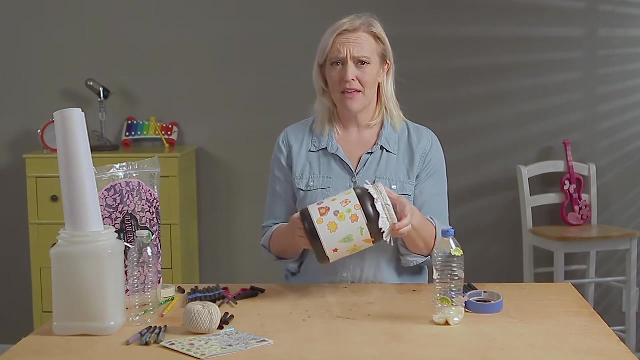 everywhere Straighten up, and there we have it. just how simple, Easy Pan flute. So that's our first one. Our second is a fun little hand drum. This is great because you can decorate and just use stuff that you have around the house. 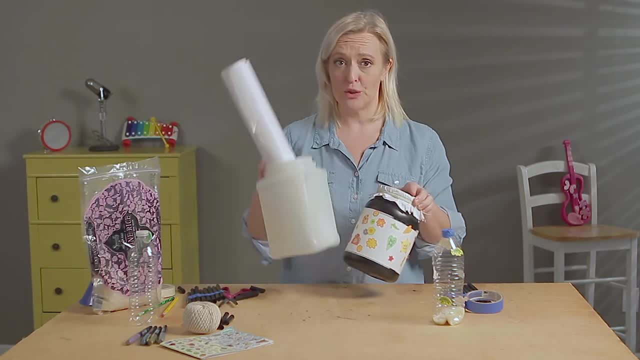 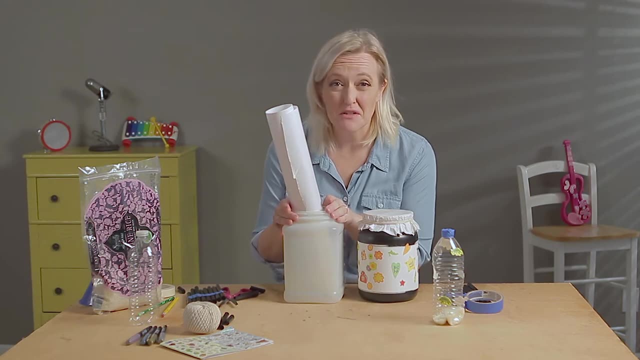 Protein shake container, or this one is just a laundry detergent container. Maybe you have a coffee can, So you just need a container. guess what? you can even use your Tupperware- And either parchment paper- this is freezer paper, just something that can go across the table. 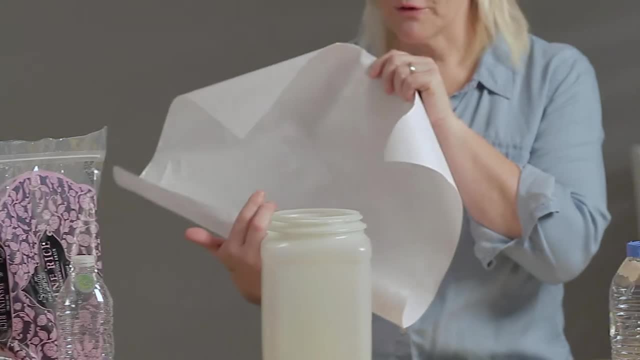 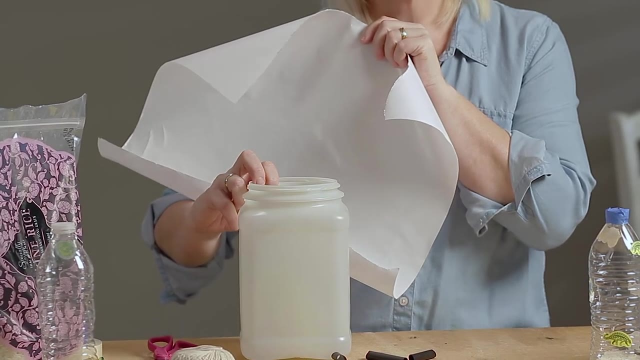 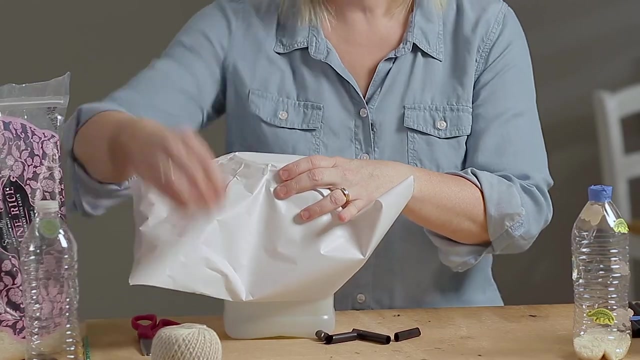 Now some people will cut the circle first to fit over the top, but I always have a habit of getting my circles wrong, Whoops. So I just tend to do it this way. I like to put my paper across and squish it down. Grab a rubber. 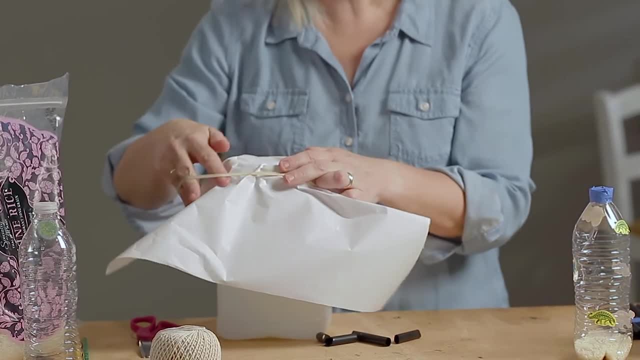 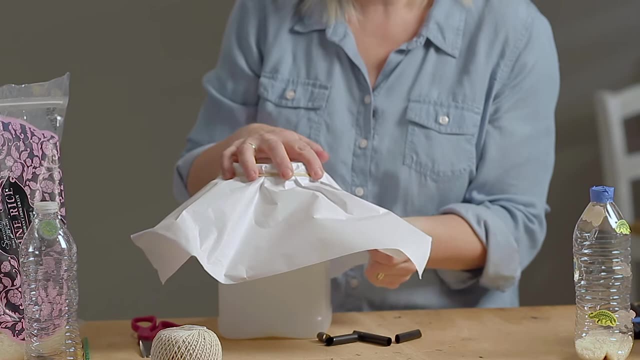 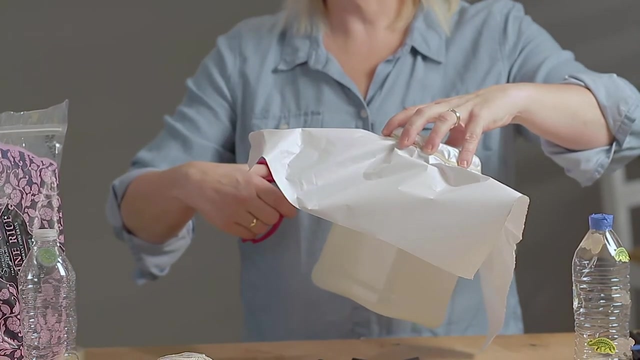 band and fit that around the top, Put it in and pull it down a little to try and make a nice little circle And make the top taut, And that's what we want. This is where I'm just going to get my scissors now and cut off the excess can. 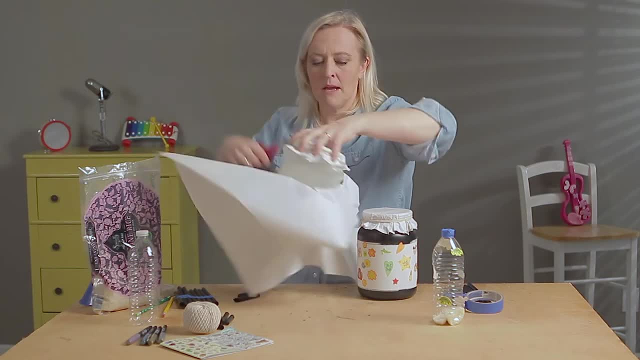 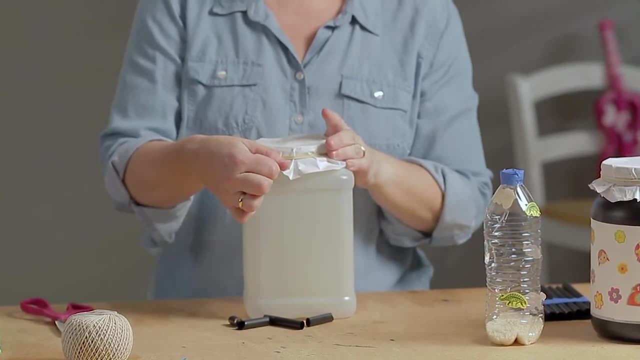 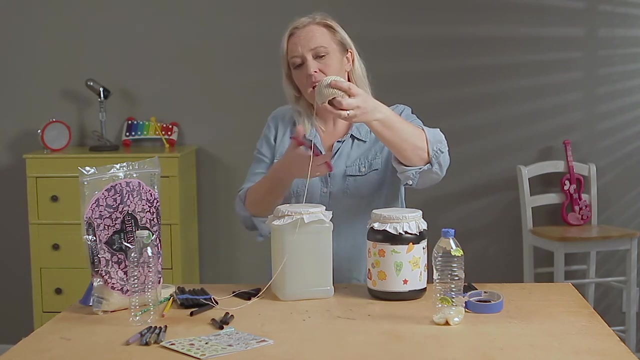 There's about 30who needs to be taught. Be you guys in the room, And this is just to help keep it tight. Cut a good length, because we can always cut the excess off. Get that done And we're done. Just kind of bye-bye. 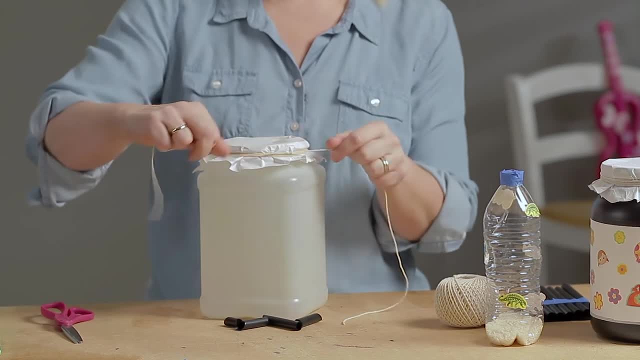 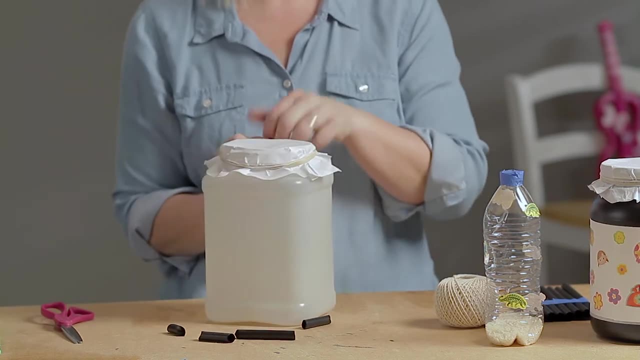 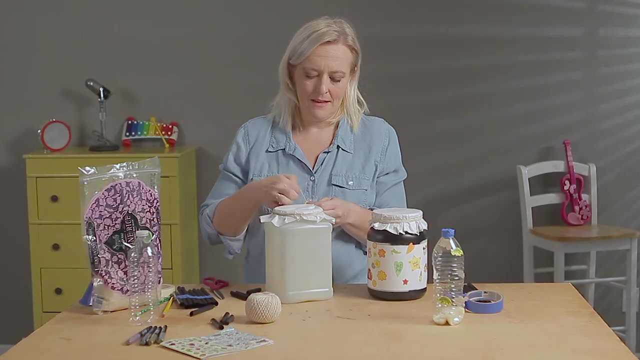 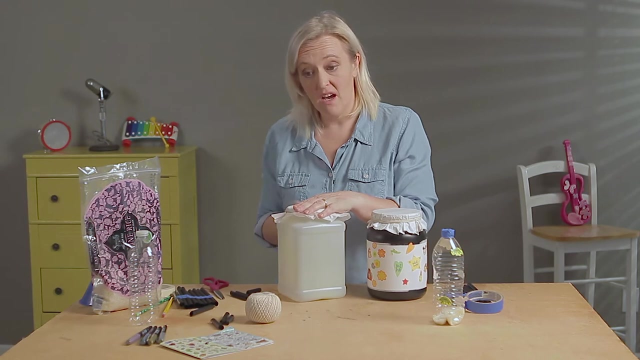 Bye-bye Dinah, And I like to wrap it around. I like to wrap it around and pull it in tighter, Knot it off, cut off the excess again, just pull again to make it tight. And this is where we really have our drum. 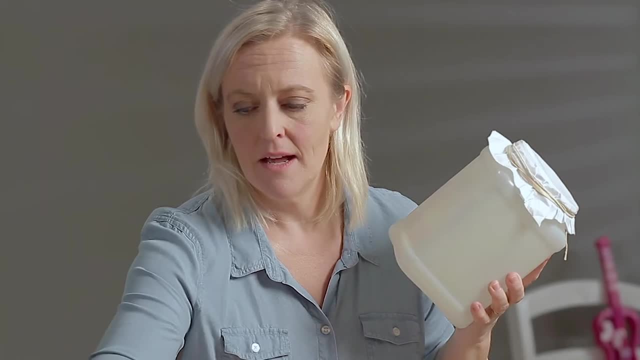 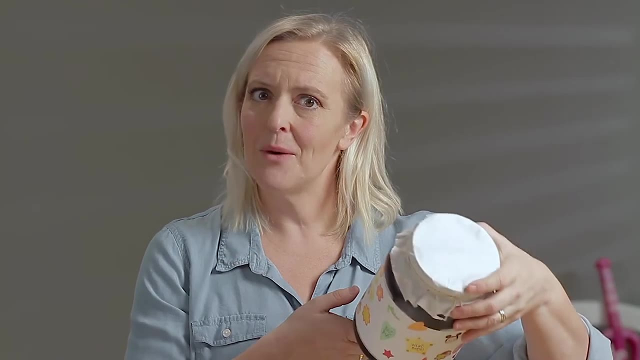 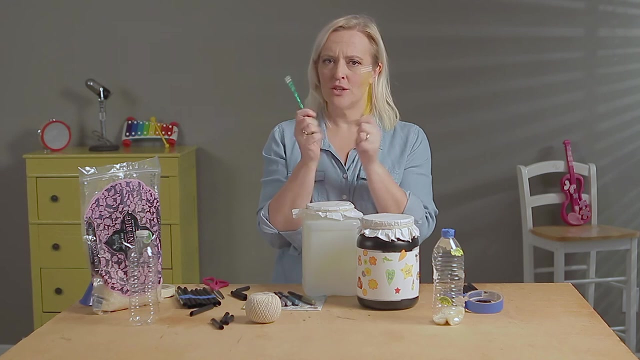 It's a bit boring. This is where stickers come in. some fun markers and let your children go to town. This is what my girls did and they had fun with it. And now we have this hand drum. Of course, you can play it with your hands as a hand drum or two unsharpened pencils. 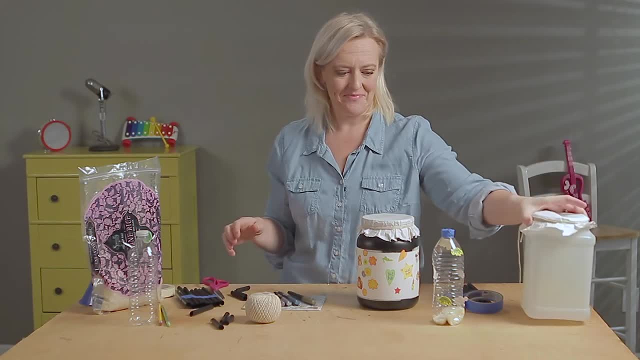 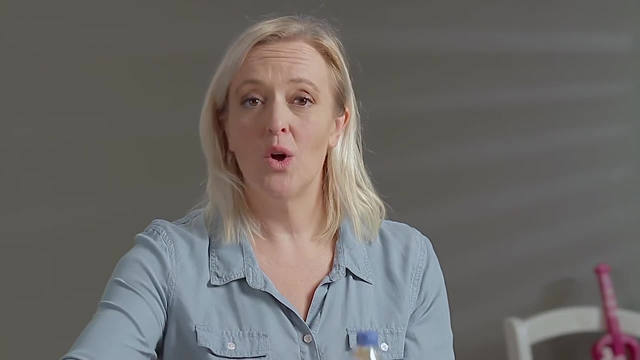 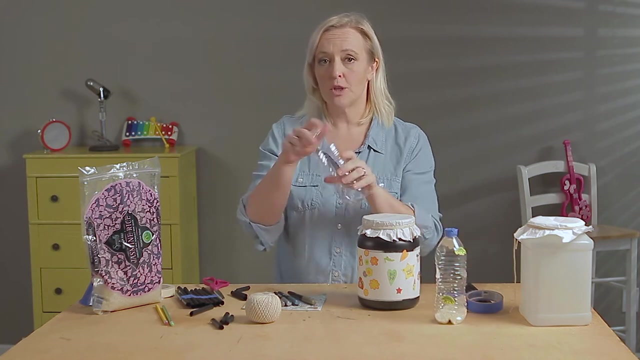 A simple, easy hand drum. And our third thing is a water bottle shaker or maraca- Again, easy. All you need is a water bottle, some rice, some tape and some things to decorate. So you will grab our water bottle. we're going to take off the lid. 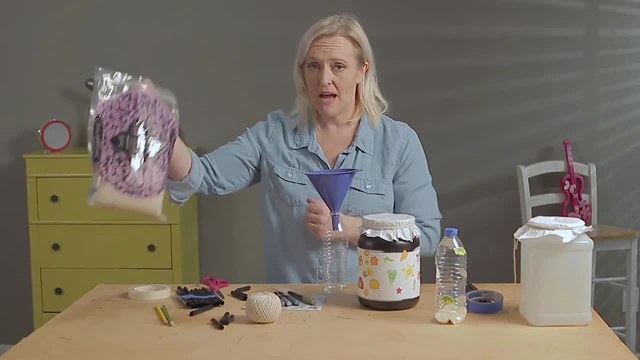 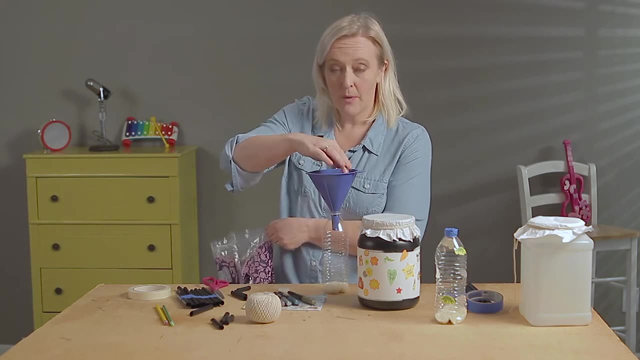 Now you can use beads or dried beans if you have them. we just have rice in the house And we're going to pour some rice in, Up to you how much. Oh, that's good. I like to do about two handfuls. 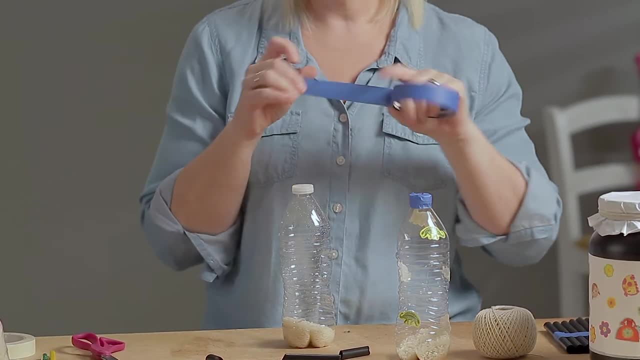 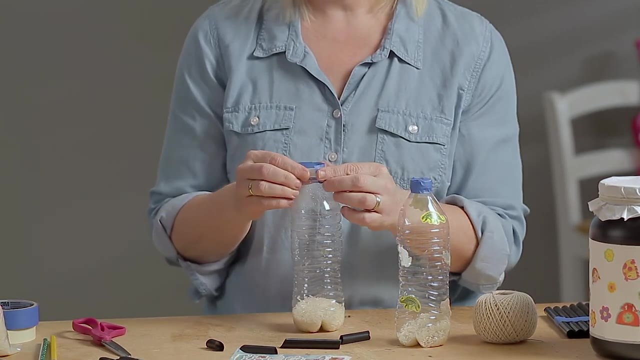 Put your cap back on, your lid back on and get some tape to seal it up. I like to do this so that a cap doesn't fall off and rice goes flying everywhere. Now, of course, to my girls, tape is not much of a deterrent. 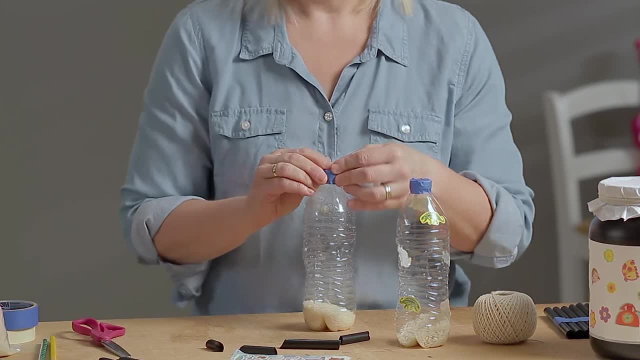 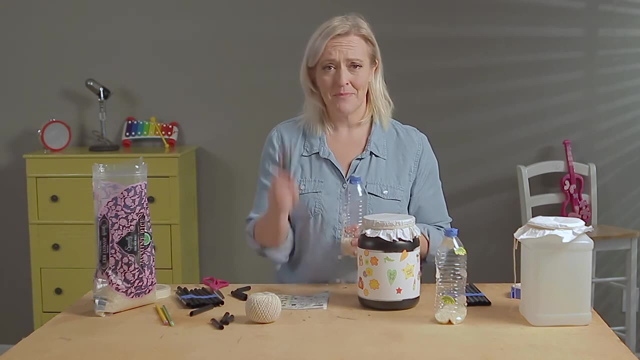 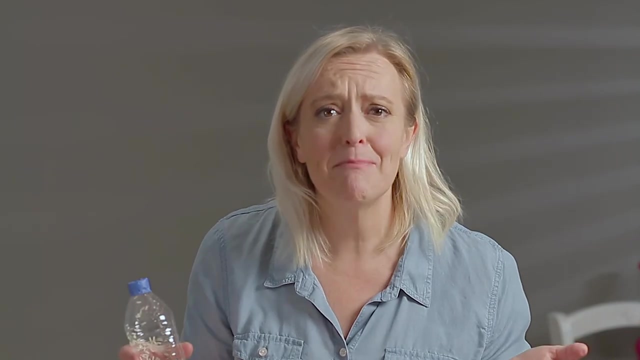 They're like ooh tape. let me take that off. But we have it And voila, Our water bottle shaker, our maraca, And again Markers, Stickers. Just have fun decorating And now you can have a family band.